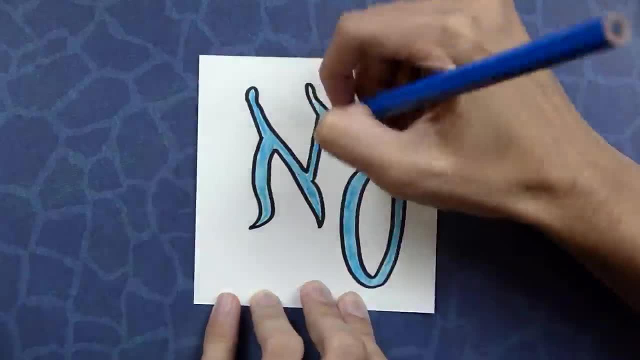 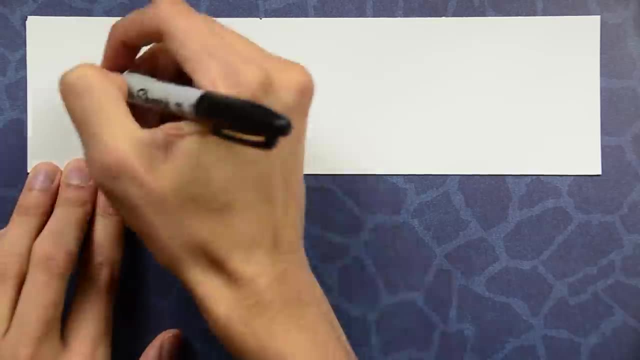 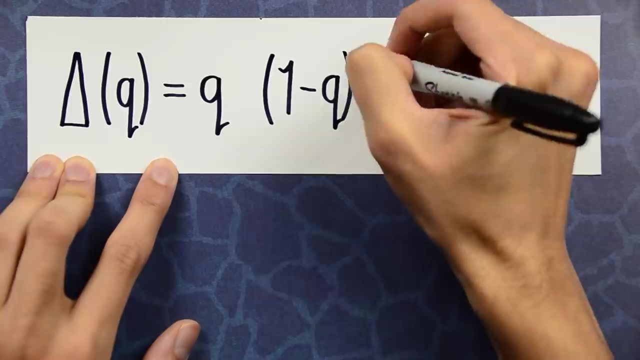 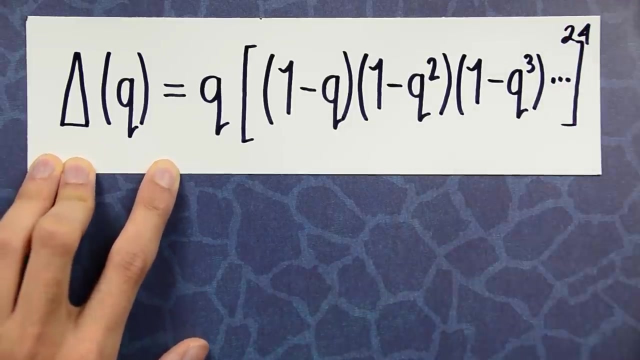 In 1916, the mathematician Ramanujan looked at the following very strange function, which he called delta, of q, q times 1-q times 1-q squared times 1-q cubed, and on and on, And then all of this raised to the 24th power. For no particular reason, he decided to multiply. 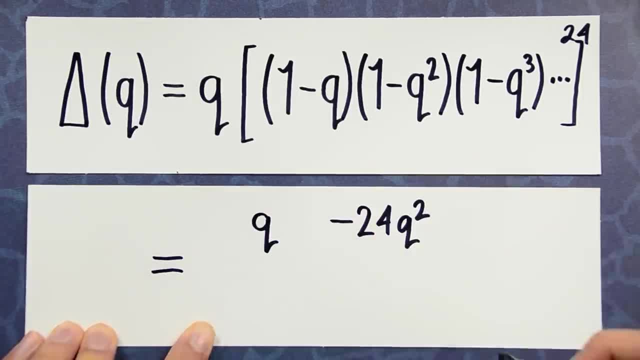 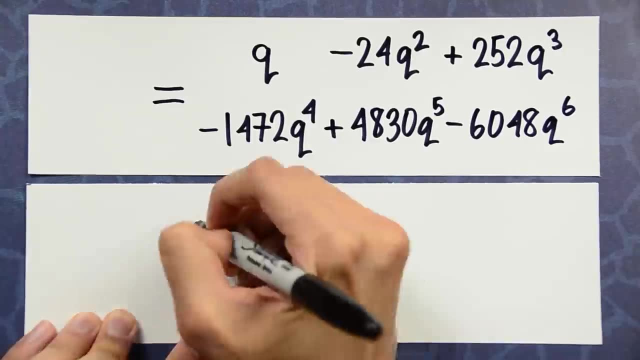 it out And when he did, he got this strange sequence of numbers. While most people wouldn't have looked twice at this list, Ramanujan noticed something very strange: If you took this number and multiplied it by this number, it equaled this number. Another observation: 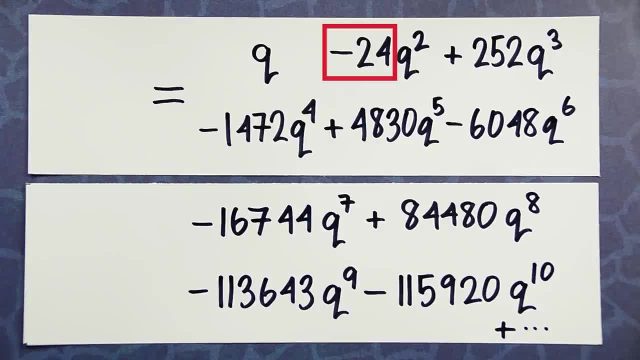 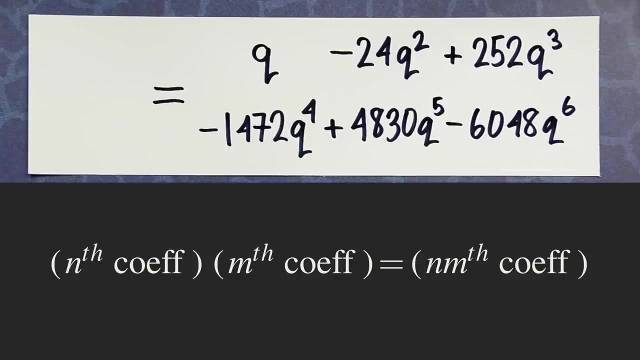 If you wrote out some more coefficients and you took this number times this number, it equaled this number. In other words, the coefficients of this function were multiplicative. The nth coefficient times the mth coefficient equals the n-nth coefficient whenever n and 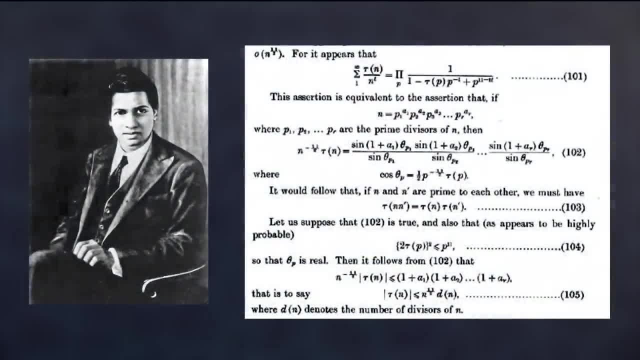 m were co-prime. Ramanujan himself didn't know how to prove this, and he conjectured it in what is now a very famous 1916 paper. What we now know is that Ramanujan's identity is reflective of the fact that these are no ordinary numbers. They actually contain some. 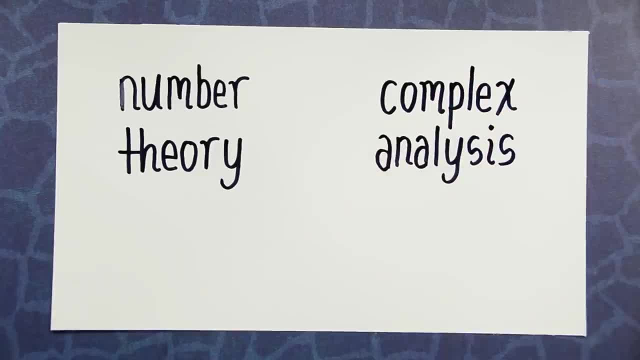 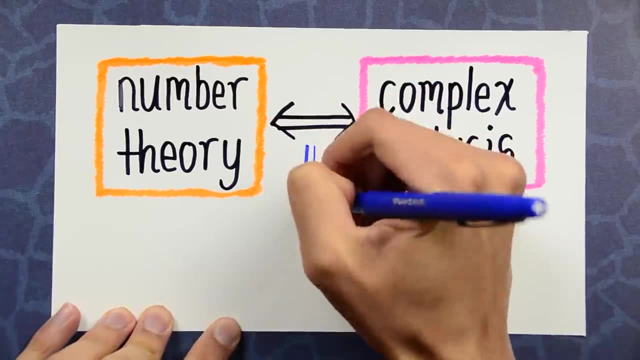 very deep meaning. In this video we'll see what the true meaning of these numbers is and how they form a bridge between number theory and complexity. We'll then see how that bridge leads to the proof of Fermat's Last Theorem. 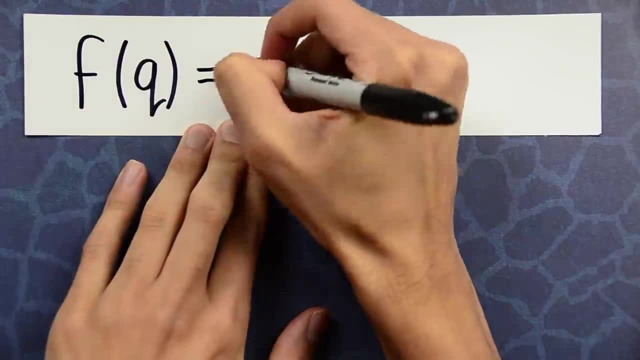 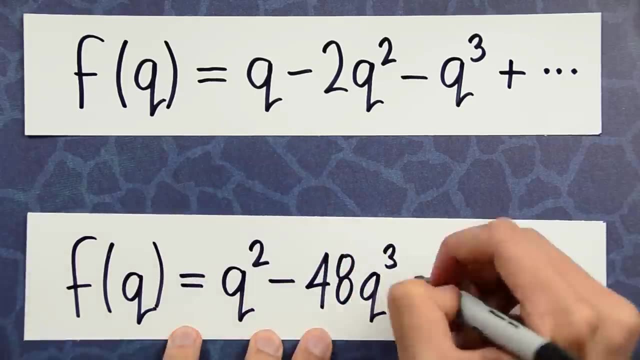 In a bit more detail. that's because the function that Ramanujan discovered is not alone, but actually belongs to a very huge family of functions that we now know are very deep. The numbers that appear in their coefficients have an interesting hidden meaning. These 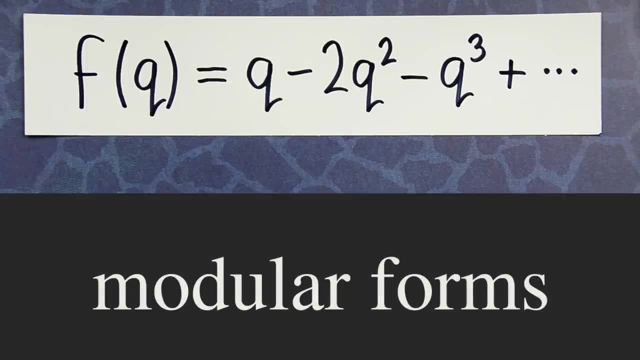 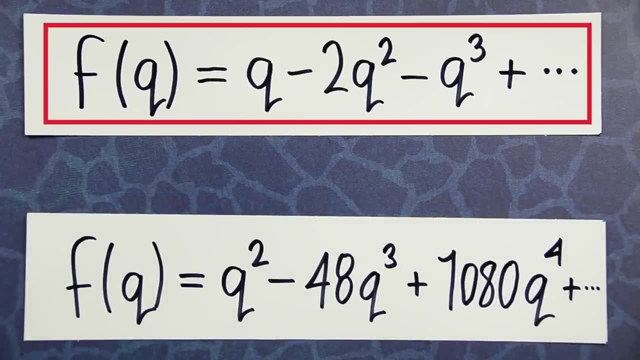 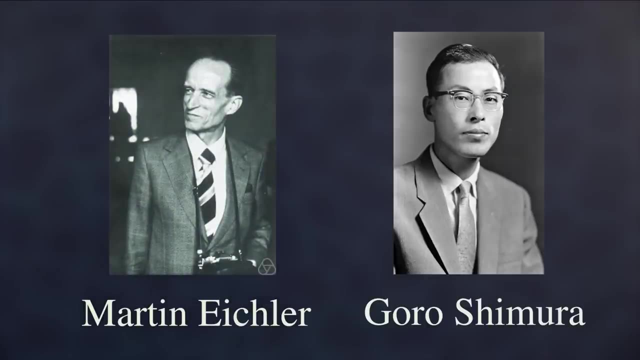 are functions that we call modular forms. This video is an intro to what modular forms are and how they proved Fermat's Last Theorem. I'll focus on this one here. Our story begins in the 1950s with mathematicians Martin Eichler and Goro Shimura. They looked 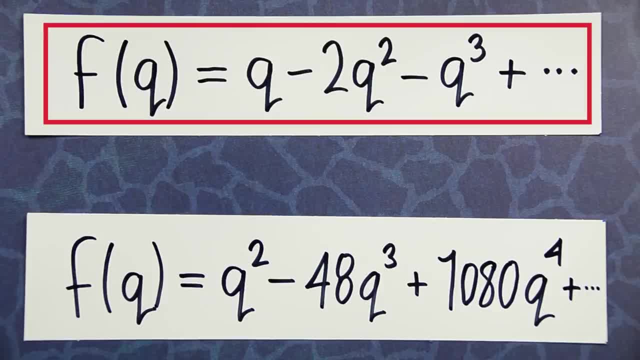 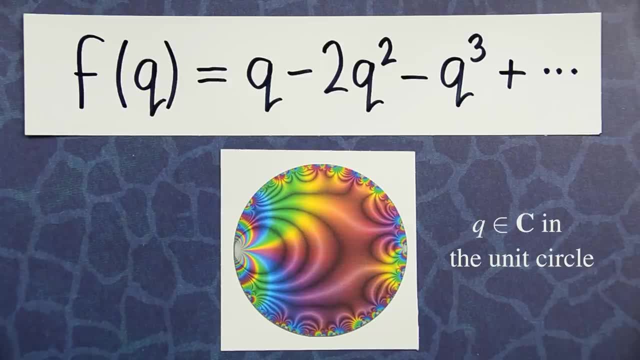 at the coefficients of this modular form and wanted to understand their true meaning, so to speak. The first key step was to visualize this function in the complex plane. Here the variable q is a complex number in the interior of the unit circle. in the complex 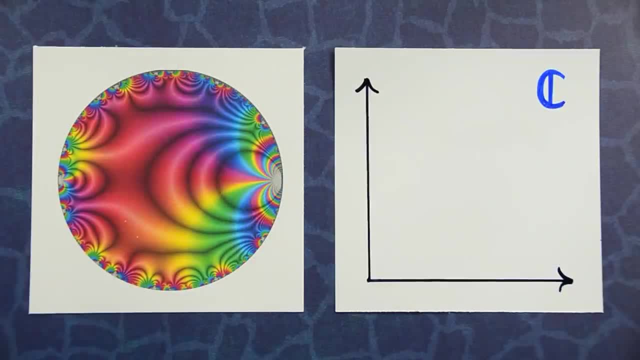 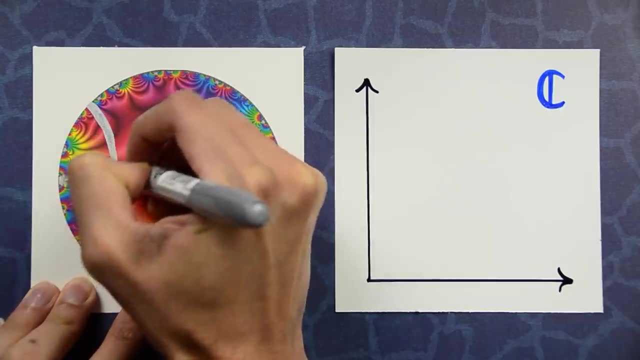 plane To find the true meaning of the coefficients of the modular form. they took a curved arc in the circle and integrated the modular form over that curved arc. That is, they added up the values of this function over the arc. That gives you a complex number. Let's plot. 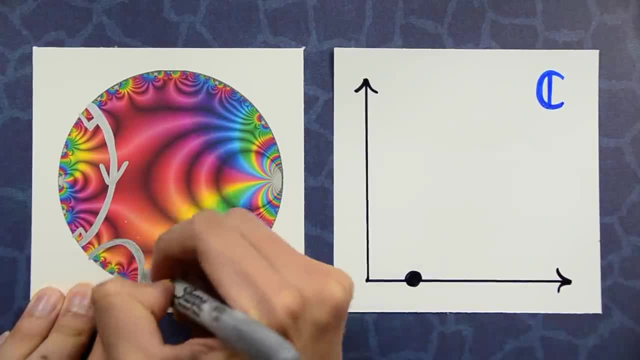 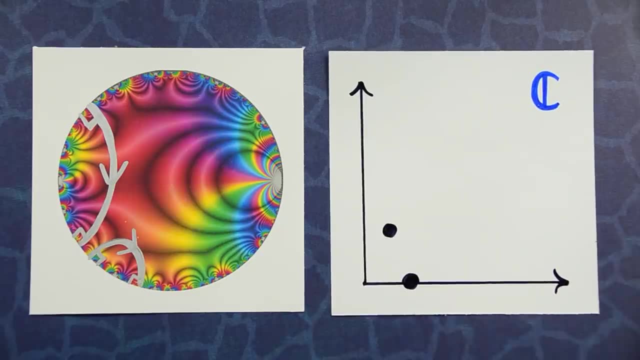 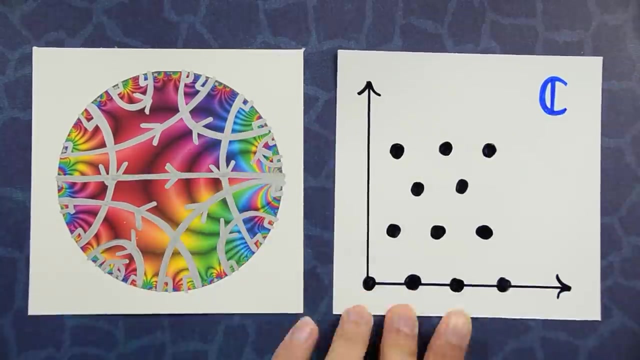 that over here on the right Now. take another arc in the circle and integrate the function over that arc. That gives you another complex number. Let's plot it on the right Now. do that for more and more arcs in the circle. Slowly you notice that a pattern is being created in the circular plane. This is the 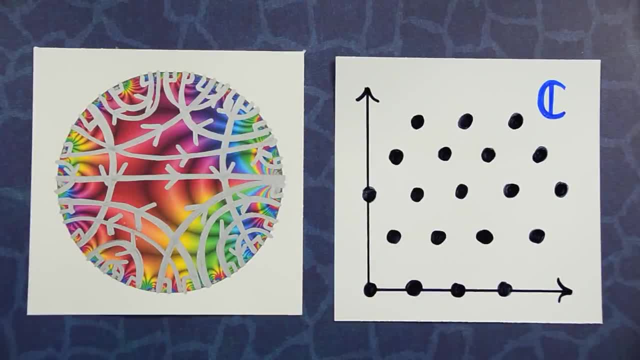 same pattern that starts forming on the right, The values on the right form, a lattice in the complex plane. The next insight is that this lattice has a very deep connection to numbered theory. To see it, it might be helpful to look at one dimension lower. Suppose that you have. 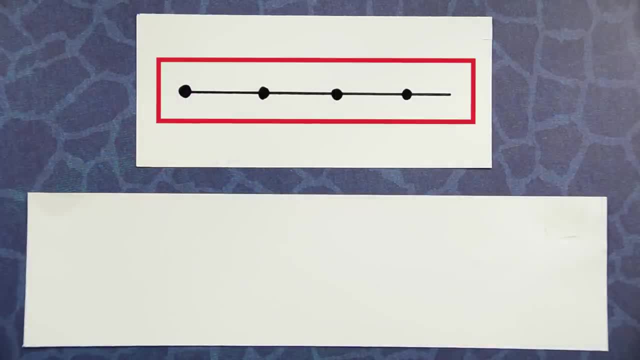 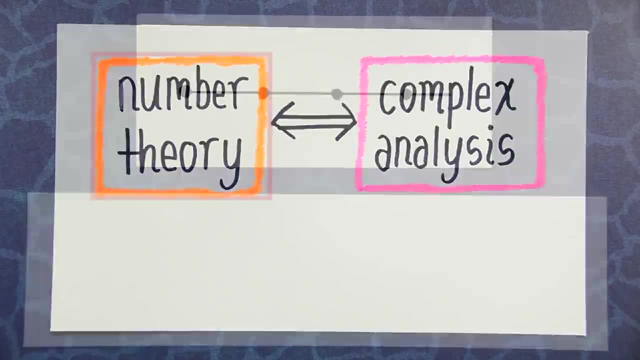 a one-dimensional lattice, just a bunch of evenly spaced dots on the number line. How do you relate this lattice to something that lives in the world of numbered theory? Well, you can do the following thing: Take a function that repeats in every portion of this lattice. 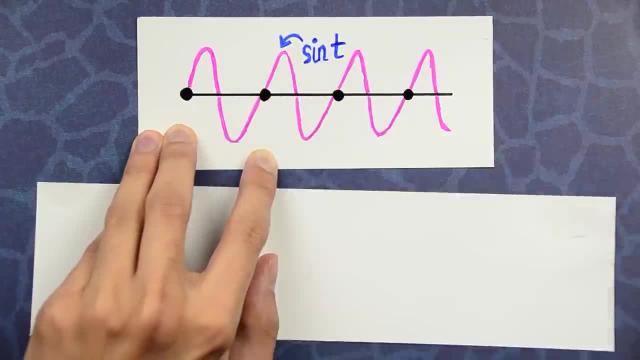 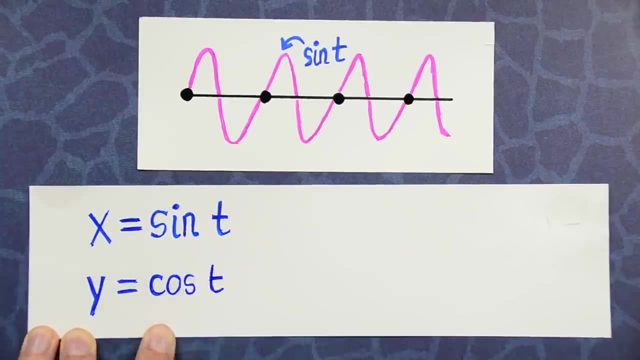 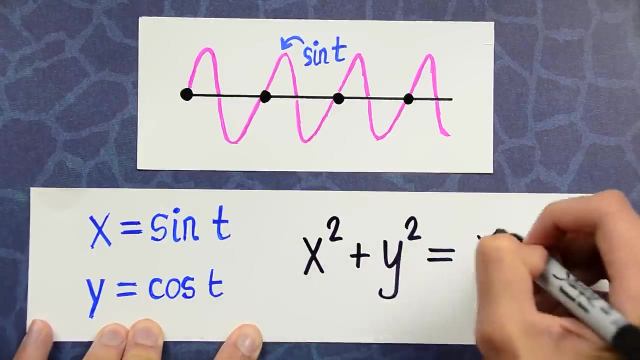 So what we've drawn is the sine function. It's periodic. Then set the variable x to equal sine of t and set the variable y to equal cosine of t And notice that they satisfy the following equation: x squared plus y squared equals 1.. So we started off with a lattice. 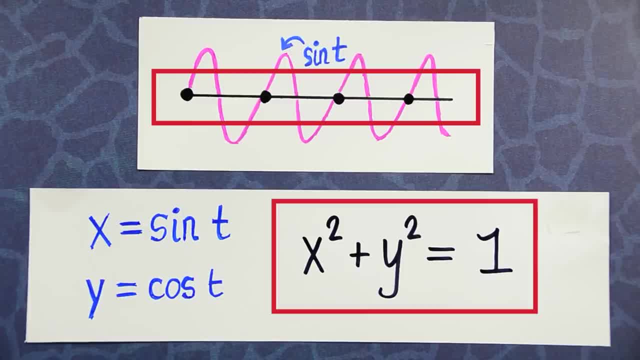 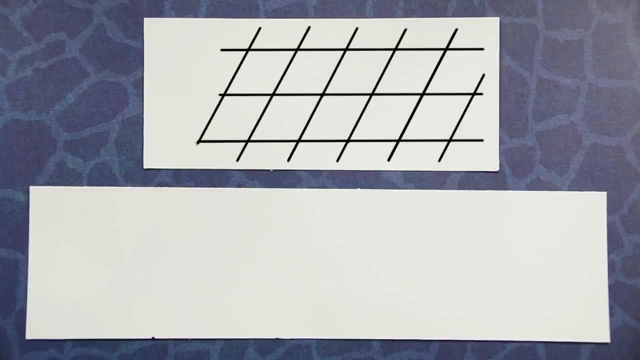 and ended up with an equation which lives in the world of numbered theory. What we'll do now is an analogous process in higher dimensions. Given this lattice, we're going to have to look at a higher-dimensional analog of sine, which repeats in every square of the lattice. 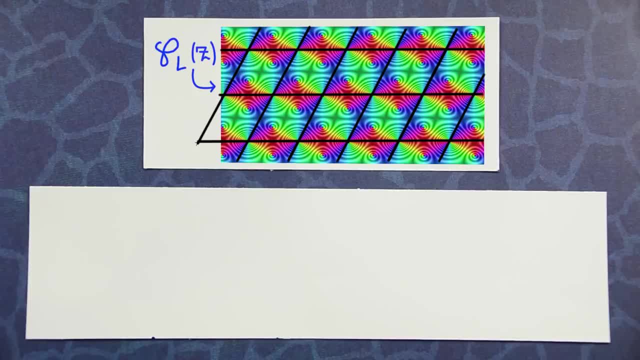 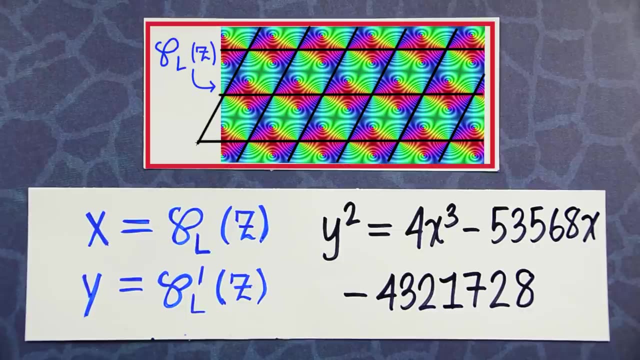 The function you're looking at right now is called the Weierstrass p function. Set x equal to p of z and y equal to p, prime of z, Then x and y satisfy this rather complicated-looking equation. So, just like before, we started off with a lattice and we cooked up something which 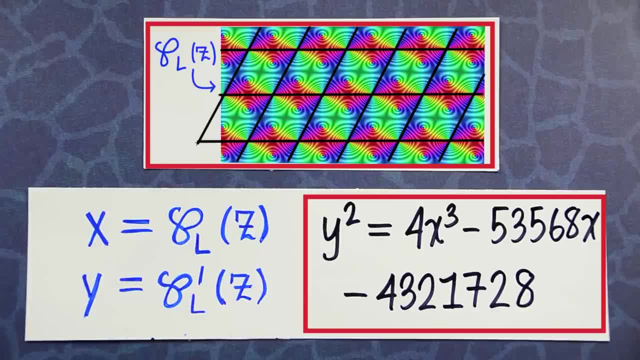 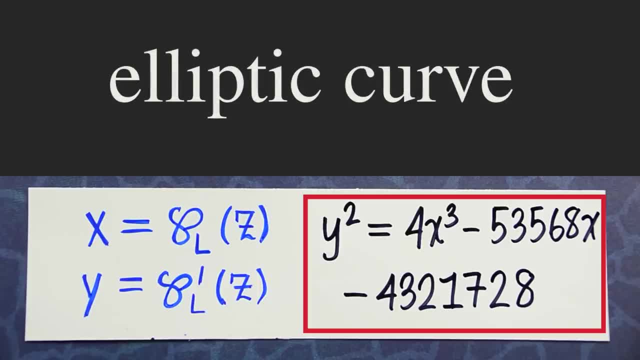 lives in the world of numbered theory, an algebraic equation. Now this equation over here is given a fancy name: It's called an elliptic curve. Let's summarize what we've done so far. We started off with a modular form From it. 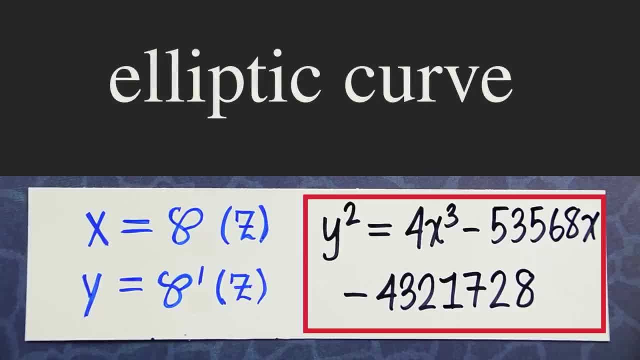 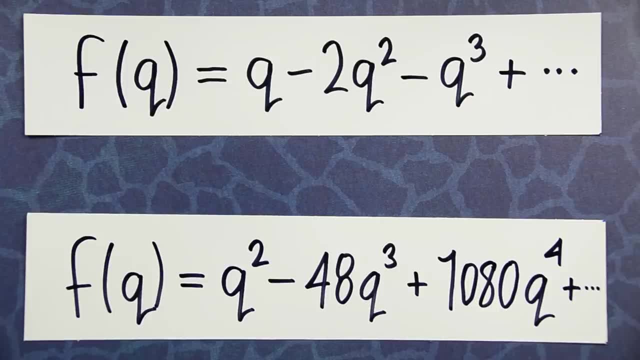 we cooked up a lattice And from that lattice we produced this equation over here, an elliptic curve. But we started off the video wanting to know what is the hidden meaning of the coefficients of this modular form. The point that we're leading up to is that they are 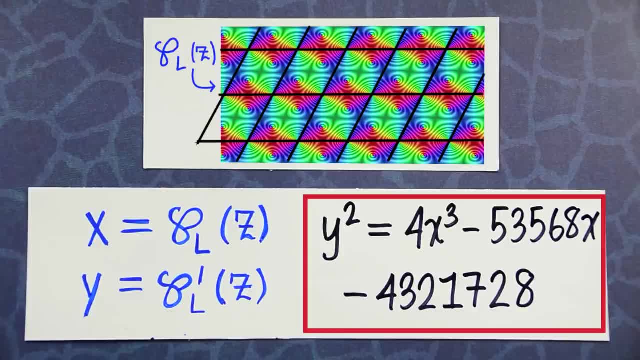 exactly reflected in the numbers. So what we're going to do is we're going to start off with an elliptic curve and then we're going to calculate the number theory of this elliptic curve. But how is that so? Well, in the world of numbered theory, a standard question people ask when: 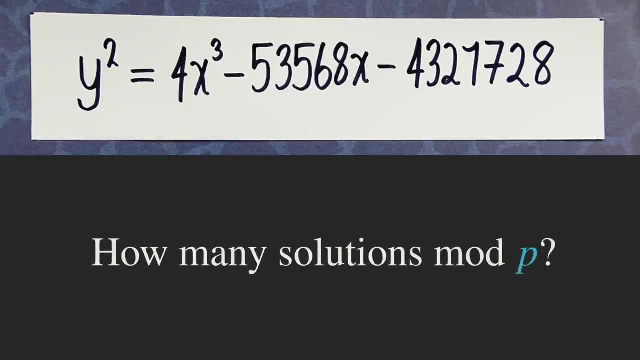 given an equation is the following: How many solutions are there to this equation mod p, where p is a prime number? For example, if p equals 5, then the pair is a solution mod p. That is, if you substitute x equals 4 and y equals 1, you'll see that the two 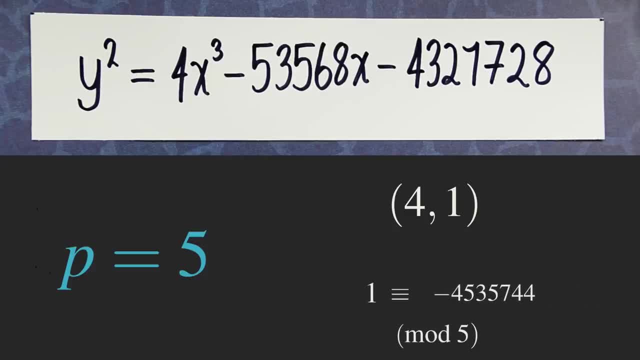 sides are congruent: mod 5.. Similarly one can check with the brute force search that there are four solutions to this equation- mod 5, listed here. We can do this for every prime number p. So for every prime number p we can count the number of solutions to this equation, mod p. For p equals 2, there. 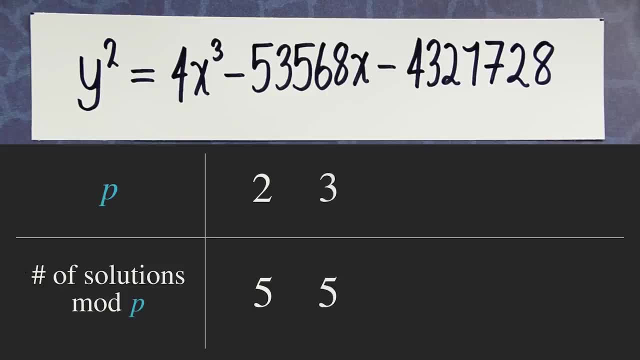 are five solutions For p equals 3,. there are 5 solutions. Likewise, you can fill this out for all primes: p Sum. Now, this list of numbers doesn't look too interesting at the moment. Here comes the magic. Instead of considering the number of solutions, mod p, consider this slightly weirder thing. 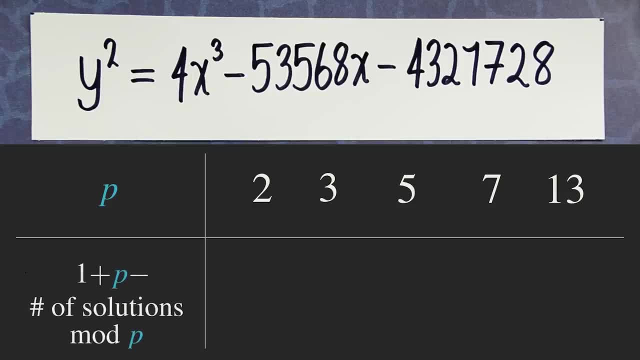 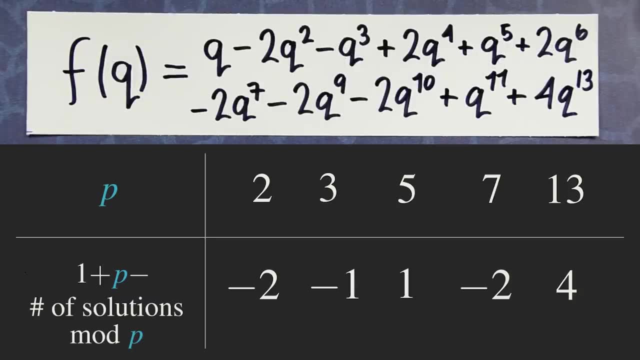 – 1 plus p minus the number of solutions, mod p. Here are the updated numbers. The point is, these numbers exactly match the coefficients of our modular form. For example, the number here is negative 2.. And the second coefficient of our modular form is negative 2.. 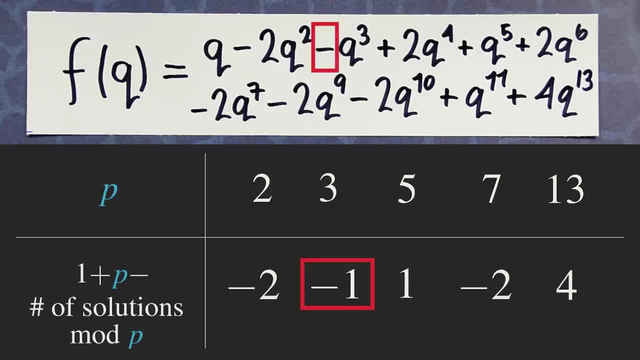 The number here is minus 1.. And the third coefficient of the modular form is minus 1.. Likewise for all the other numbers. We started off the video saying that the coefficients of a modular form have a hidden meaning. We can now see what this is. 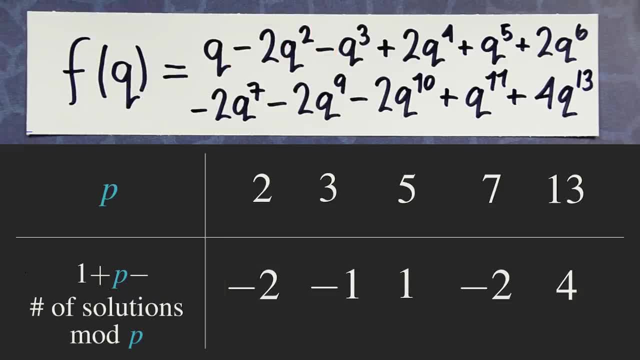 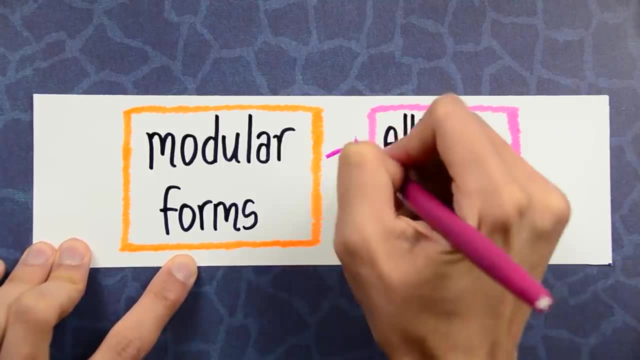 These coefficients somehow count the number of solutions to an algebraic equation. living in an opposite corner of math, They have a strange predictive power. In other words, we have two worlds: Modular forms and elliptic curves. What we've done is to a modular form, we've attached to it an elliptic curve. 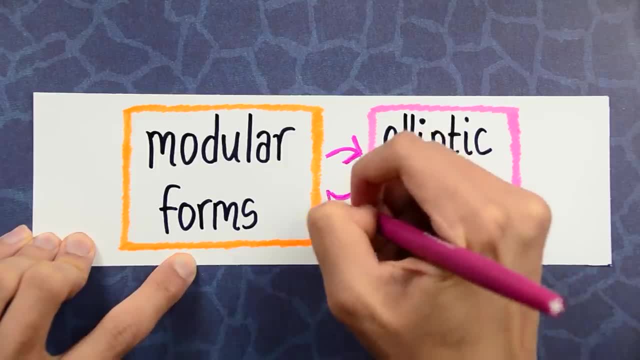 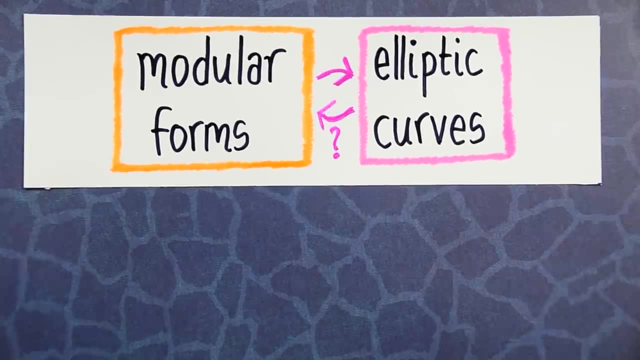 But it wasn't until many years later that people dared to suggest that you might be able to go back, That maybe every elliptic curve came from a modular form. Now, when you first hear this, a reasonable reaction is that it seems very unlikely. 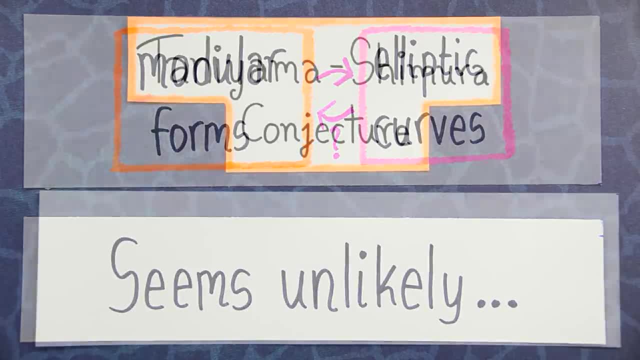 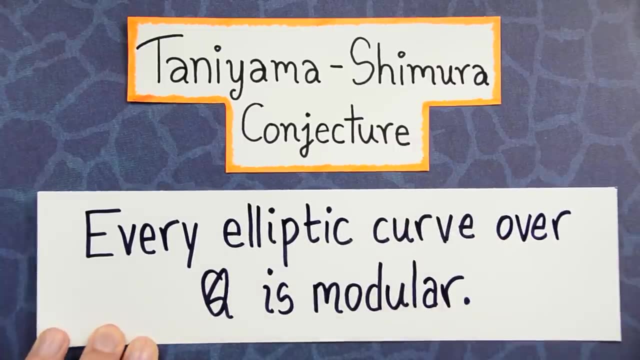 But in 1967. This feeling was formalized into a conjecture that became known as the Tanayama-Shimura conjecture. Every elliptic curve over Q is modular. That is, for every elliptic curve over Q there is a modular form whose coefficients 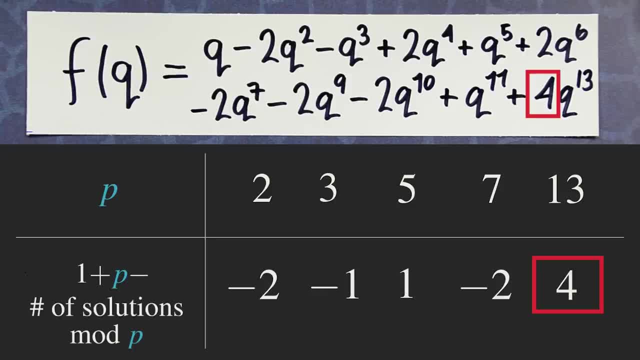 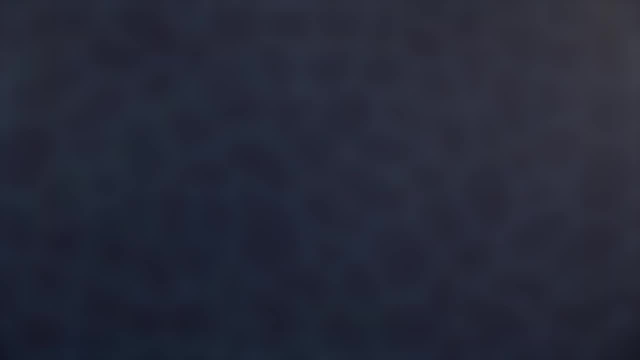 are essentially the number of solutions, mod p, to this elliptic curve. Now, the trouble with this conjecture is that nobody knew how to begin attacking it. John Coates, a very well-known number theorist, said: beautiful though this problem was it. 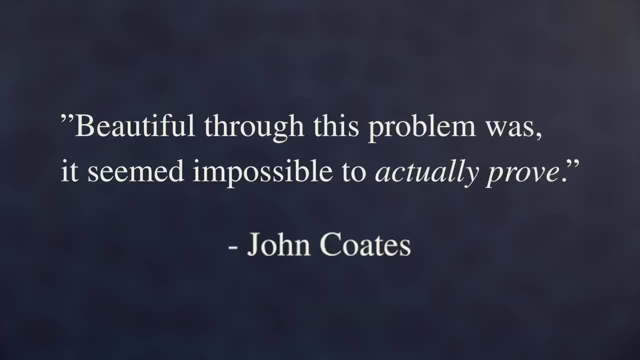 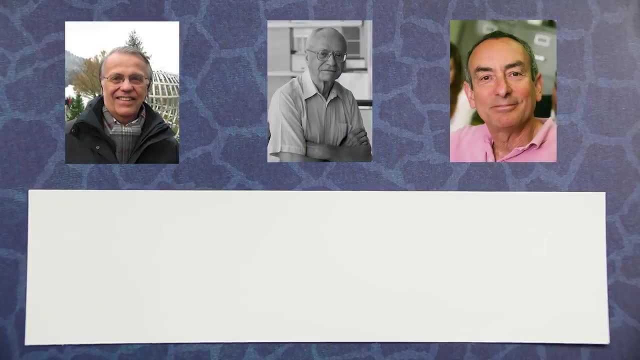 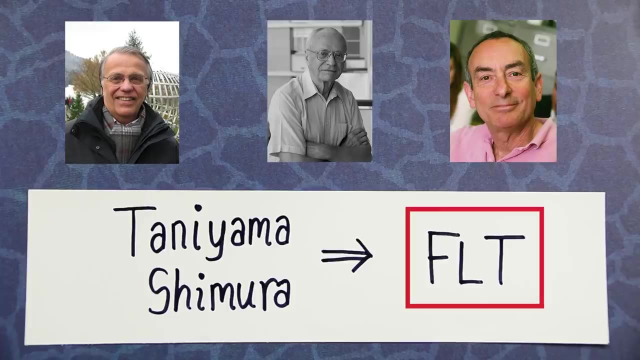 seemed impossible to actually prove. And then, 20 years later, the stakes were raised even higher when Frey Seyr and finally Ribbit showed that the Tanayama-Shimura conjecture implies Fermat-Las theorem. There was a joke that time that this was reducing one impossible problem. 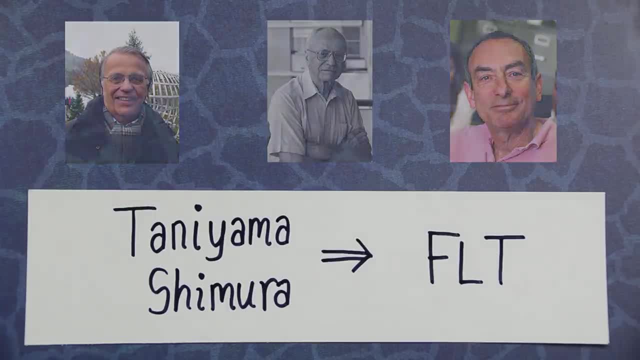 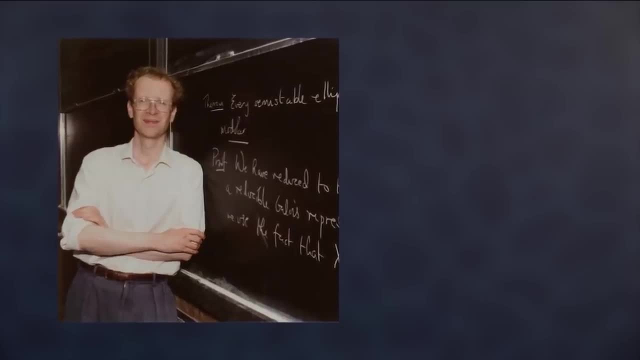 to another, equally impossible problem, But unbeknownst to the rest of the math world. somebody had been working in secret to prove the Tanayama-Shimura conjecture for 7 years, And so the answer was clear: No. 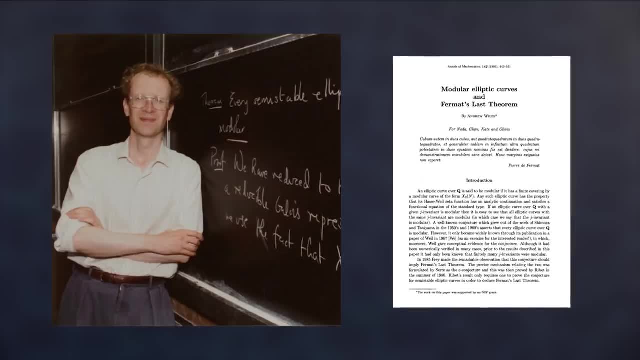 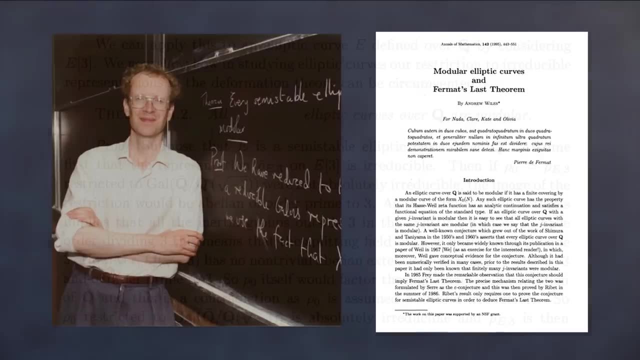 Not really. In 1994, Andrew Wiles announced that he could prove enough of the Tania-Mashmur conjecture that Fermat's Last Theorem would then follow. Specifically, he proved the following statement: Every blank elliptic curve over Q is modular. 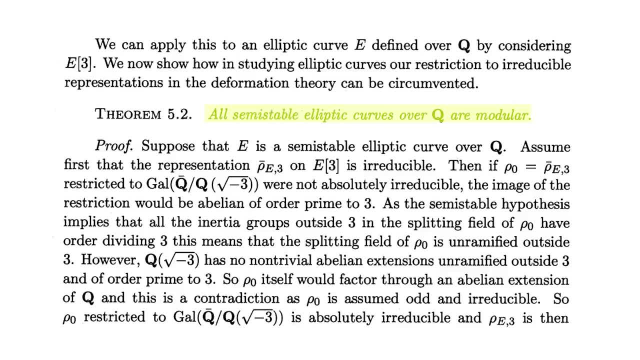 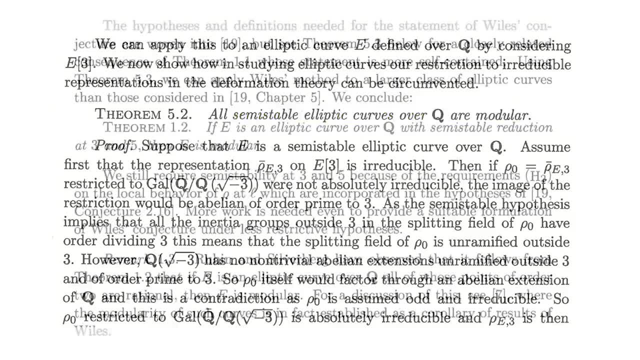 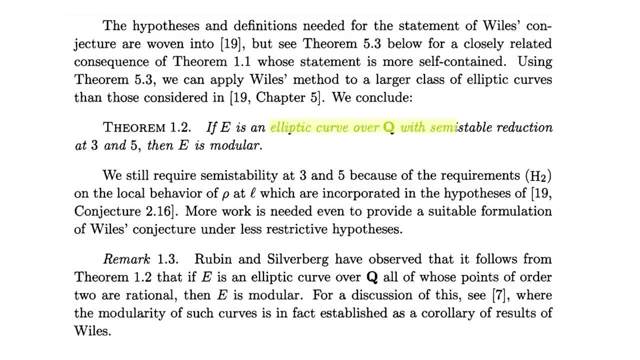 The blank over here is an adjective- semi-stable, and it was known that this statement was enough to prove that Fermat's Last Theorem was true. Slowly, slowly, in the years after people started removing conditions on the theorem, So the Tania-Mashmur conjecture was then proven for all curves that were semi-stable. 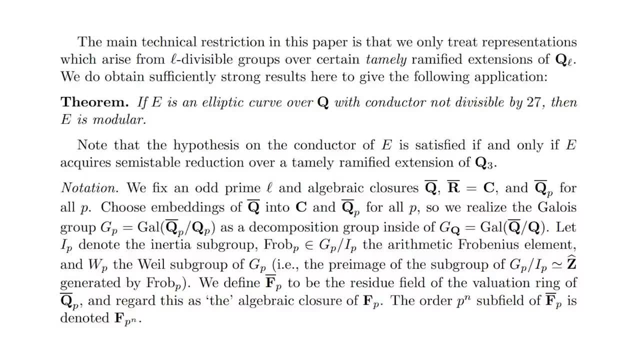 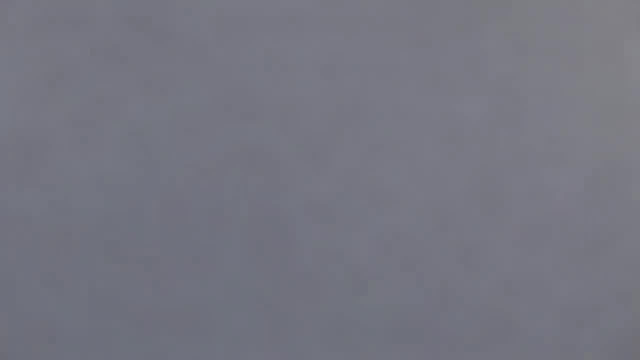 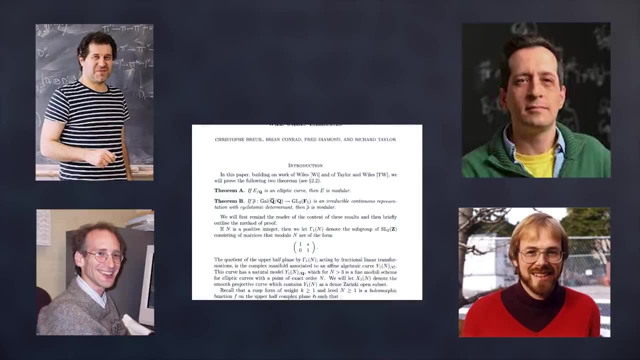 at 2 and 3.. Then it was proven for all curves satisfying an even weaker technical condition. And then, in 2001,, the full conjecture was proven by Breu, Conrad, Diamond and Taylor, And thus a theorem that first seemed impossible to attack just 40 years later, was completely. 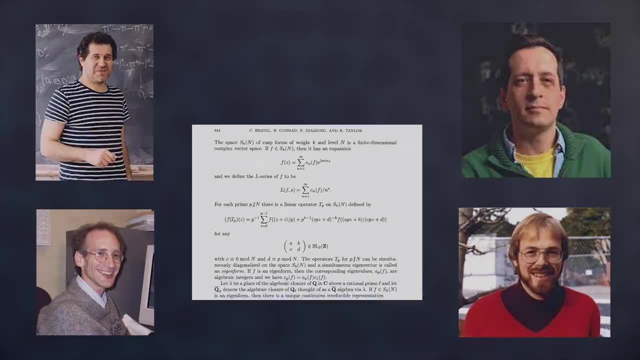 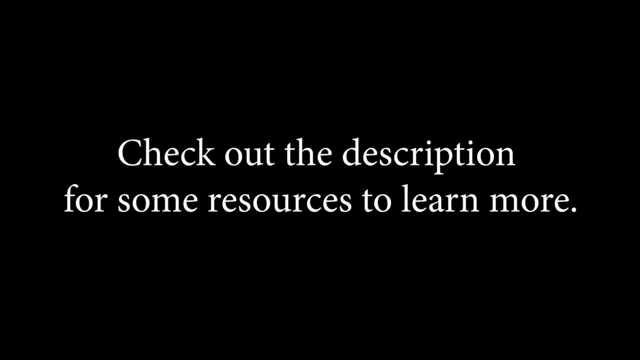 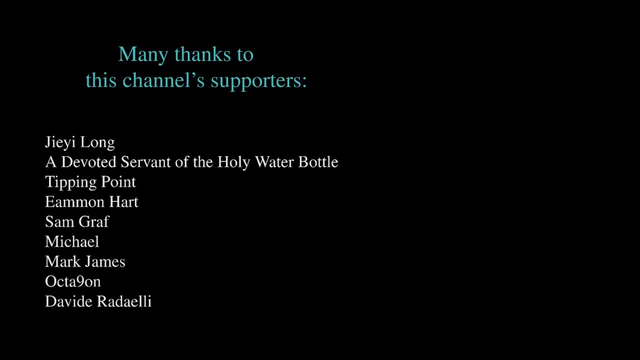 solved. That's all for this video. With that, I hope you enjoyed this video. With that, thanks for watching and I'll see you next video. Bye, bye.